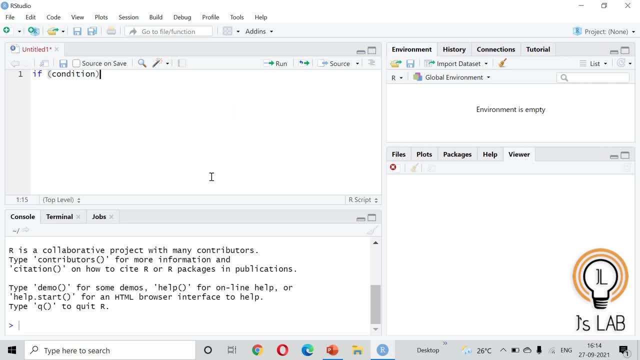 condition. Write the condition, then call you bracket. Okay, inside curly bracket you need to write what you need to do, Okay, what do you need to do? Okay, what do you need to do So that will be executed? and if it is, if you want to go for an. 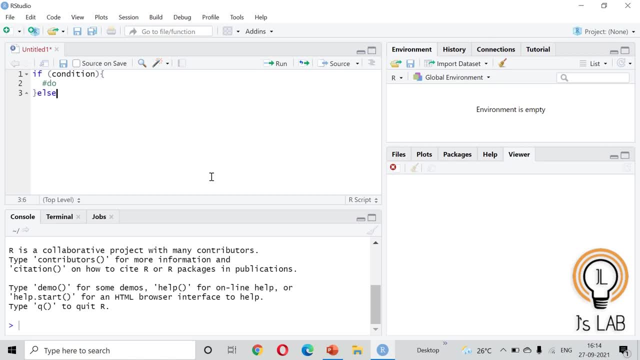 else statement, then you should add an else. Okay, else what to do? Else you open a curly bracket and close that one, Else what to do? Or you can use if chain also. Okay, if and again and if, etc. Okay, we will see one example with an example. Okay, first of all, we will give value of x as 3.. 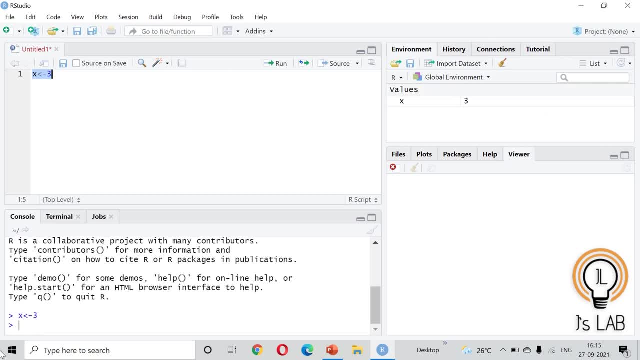 You give that as 3.. So you run. So if you type the value of x as 3, then it is. Now we are going to use this simple example. If condition is x greater than 3.. If- sorry, if x greater than 5, then what to do? Then you need to provide, you need to add y should. 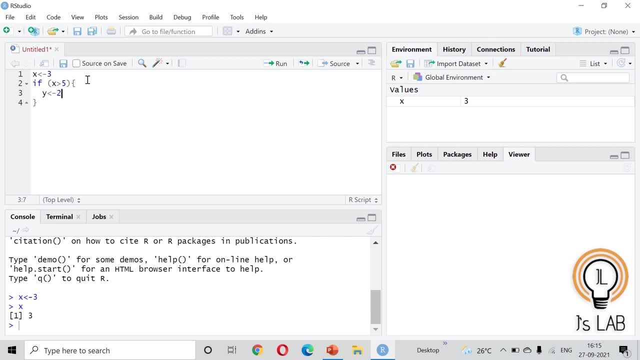 be given a value 2, for example, Okay, Else else is given a value 3.. Then what do you do else? give the value of y as 8, okay, so now, if the x is greater than 5, then y will be assigned with a value minus 2, and if- and in another case it will be assigned a y will. 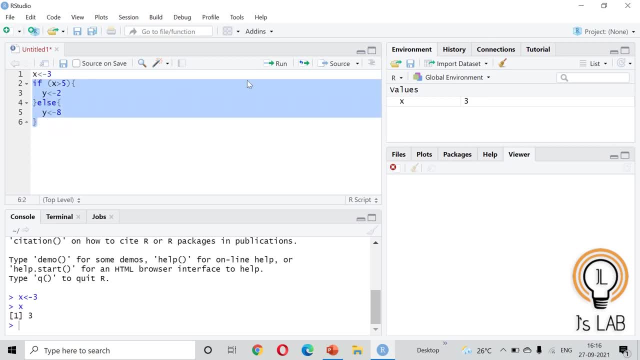 be assigned a value 8. okay, so we will run this program and run this program run. okay. now see if you, if you type the value y, you can see that it is 8 because y, x is not greater than 5. then it will say the l statement. okay, so we will. first of all, we will change the 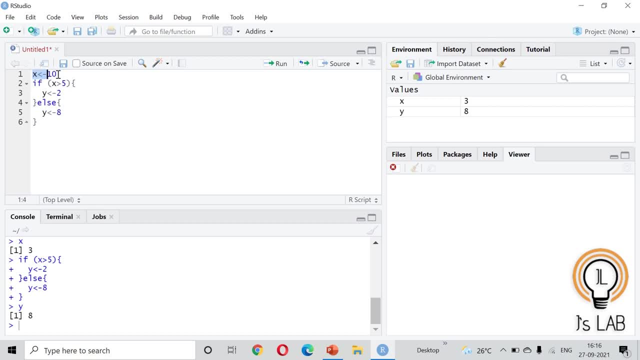 value of x to 10. okay, so x value of x is 10. we will run that one. okay, so x is given as a value 10. so it is clear it is 10. now if you execute this, if l statement, you can see that y will be assigned, you will get the value of y. y will be assigned a value 2 because 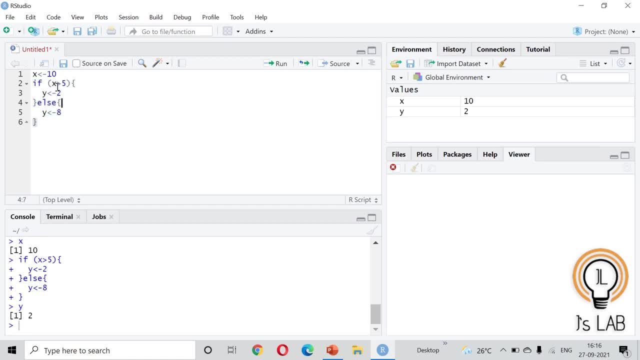 x is not greater than 5.. x is greater than 5, so first condition is true. okay, this is the if l statement. okay, so else is not necessary. you can go for x less than 3. okay, you can put some value. z should be given 9. okay, some example: less than 3. okay, so here, if you execute this one, execute. 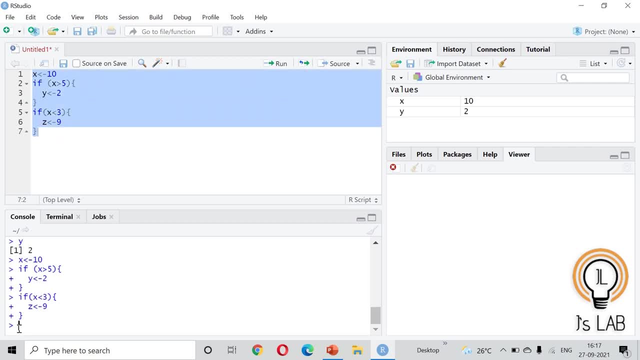 this program. so okay, execute the value of y, x, value z: no, z is not there because x is not less than 3. okay, so you give the values 2 and we will check. yeah, okay, then if you run. okay, z will be there, z. z will be given 9. okay. 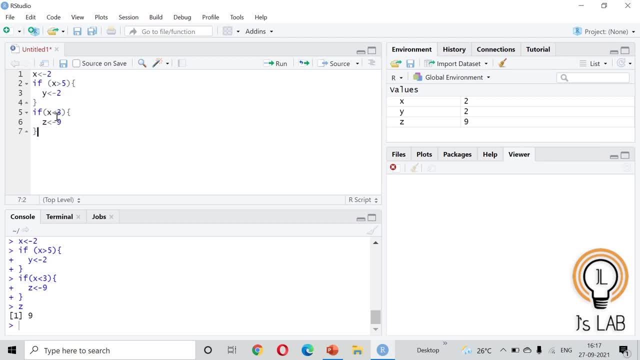 that second if is also worked, okay, so else is not a necessary one. if you want, you can use that, okay. that is if and if. l statement in r now we will see for statement for: okay. for also the condition is same. for then, inside bracket you need to provide the condition. 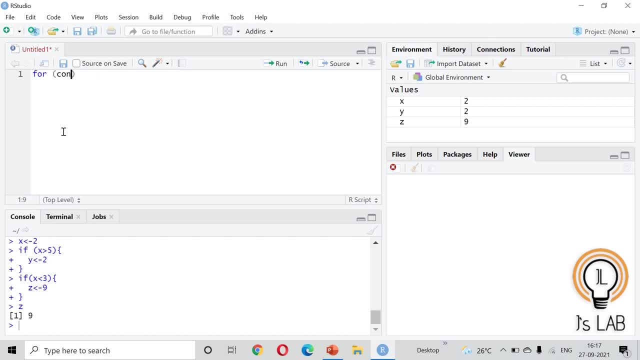 what is the condition? and no, what is the condition for looping? it is used for looping for a certain number of time. okay, for condition is given and in curly bracket, you need to do do something, what you need to do. okay, now we will see some examples. for one simple example is you need 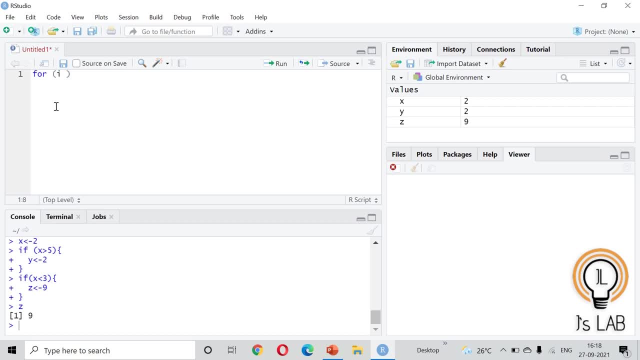 to. for condition: is you, i in 1 to 10.. 10, okay, 1 to 10, print i. this is very simple example print i. so what this will do is so it will take print i. so 1 to 10. it will say this: i will be looped from 1 to 10. okay, so first of all, 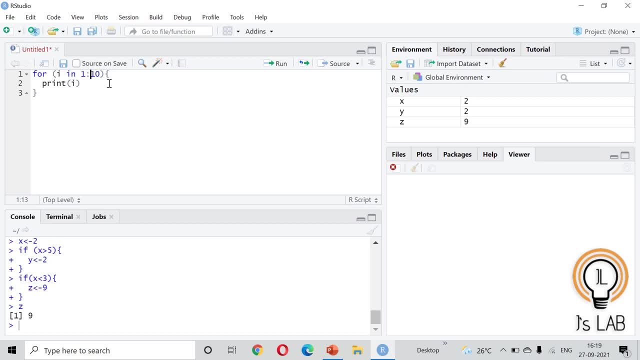 in the first step, i will be given value 1, then it will go inside the bracket it will print i, then it will loop around for 10 times. you will see that one. so front, you can see this from 1 to 10. it will be looped. okay, so you can do instead of print. you can do something here if you want to. 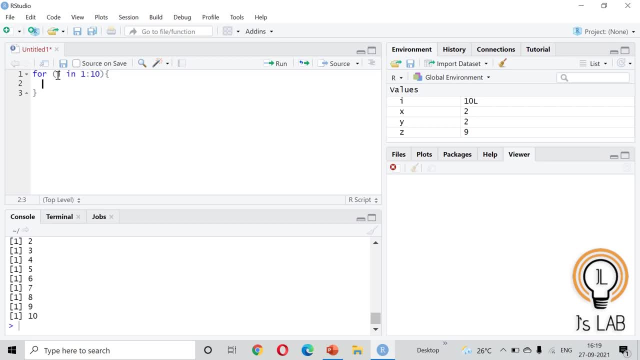 execute something that also you can do. so now you can. it is clear that this is looped for a certain number of time. okay, that is one example. go for another example. so i'll put some characters. put some characters: c, a, b, c and d. okay, so we'll run that one. okay, so x is given some values. 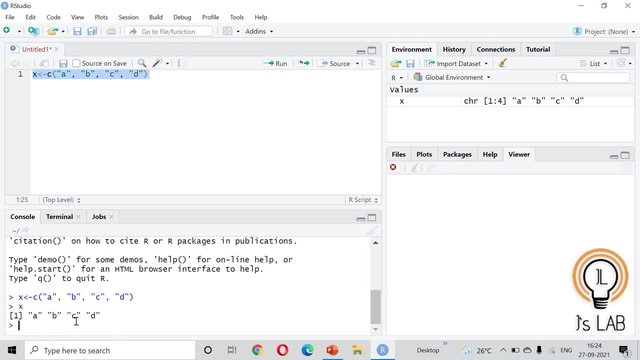 you can see here x is given four values. now we can print. okay. we can use the same example for okay instead of i. you can do any letter. you can do okay for a in one to four. sorry, curly bracket close open and in the condition is you need to print: print what x. 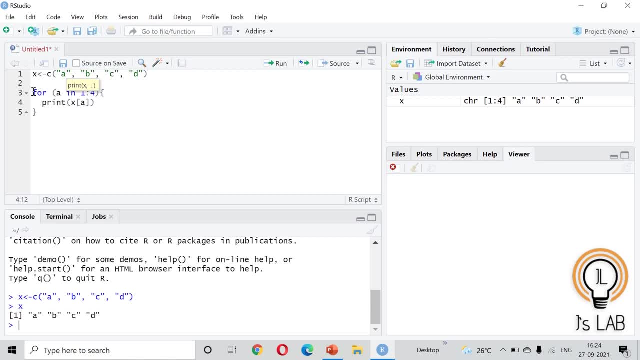 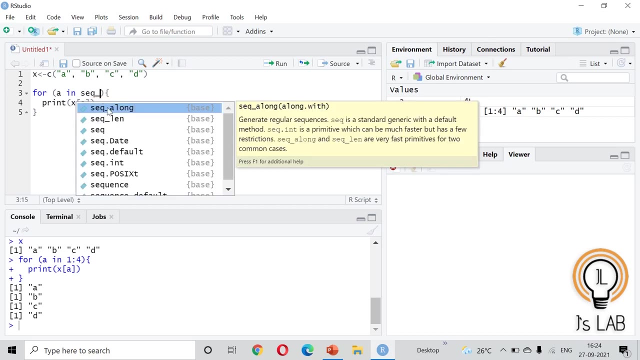 the ath term. okay, x, so it will print a, b, c, d. you can see that a, b, c, d is printed. okay, so each value. that is one thing. now we can change another thing. for a in, will you seek along, seek along? okay, so you can see: seek along, print that, run that one. the same thing. that means. 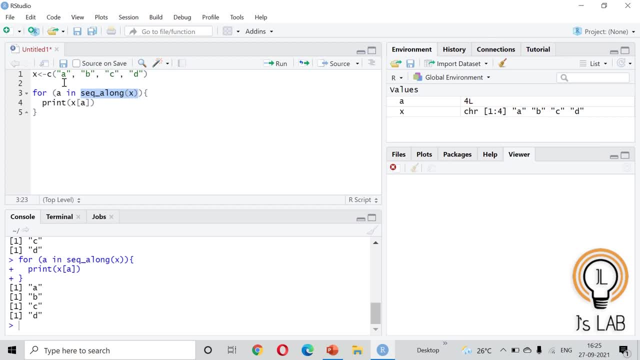 seek along means it will count number of elements: one, two, three, four, okay. so this loop will be continued for four times. the first case, a, will be one value, one, then two, three, four, okay. and the first, second, third and fourth term will be printed out. okay, that is the case of for loop. we look at another. 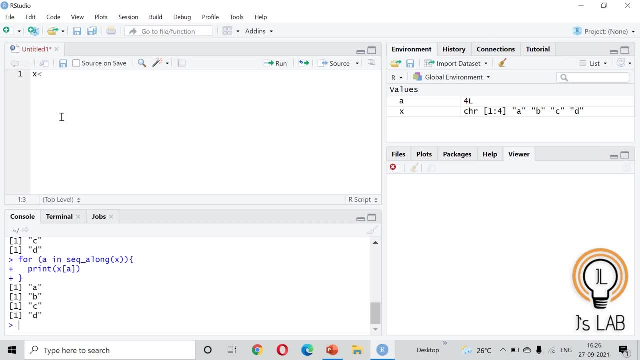 example for for loop. okay, in which for loop can be used inside one loop, inside another loop. one loop can be for loop can be used inside another for loop. okay, for that i am introducing a matrix. okay, a matrix of matrix using values one, two, six and, uh, two row and three columns. okay, so we'll uh run that one, okay, so. 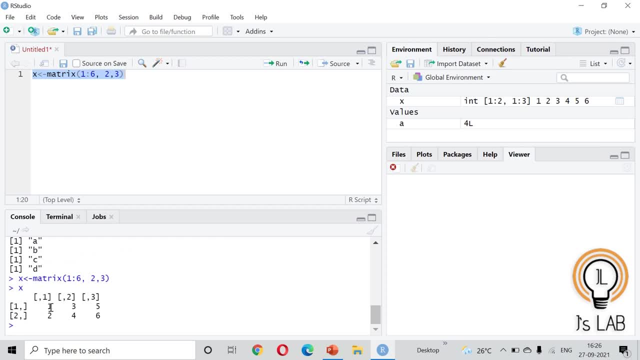 the new x value is. we'll put the x value. you can see here: one, two, three, four, five, six, two rows and three columns. okay, we introduced a matrix. now we'll uh the for loop for a in i: okay, i. in. sequence length: okay, seek length: len. 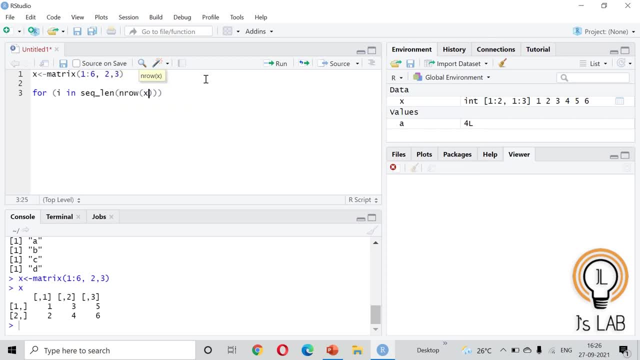 len n. row of x. okay, n row of x. so for that, what do you need to do? open the curly bracket, then right, then inside that one you are putting another for loop for j in seek len len of x of n. call x: okay. number of columns in x. 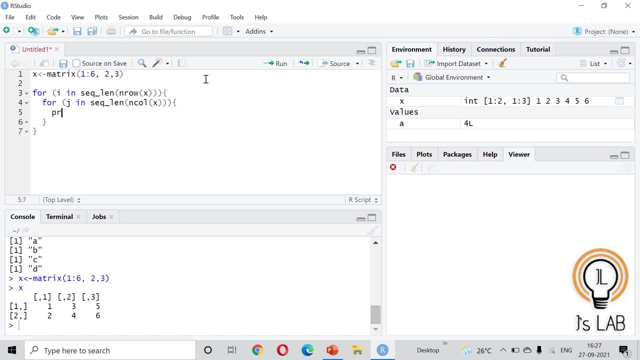 and for that you need to print print x of i term and i term i throw and jth column. okay, so what it will do is, first of all, i in c length of n row, so number of rows will be two. okay, so it will uh take. 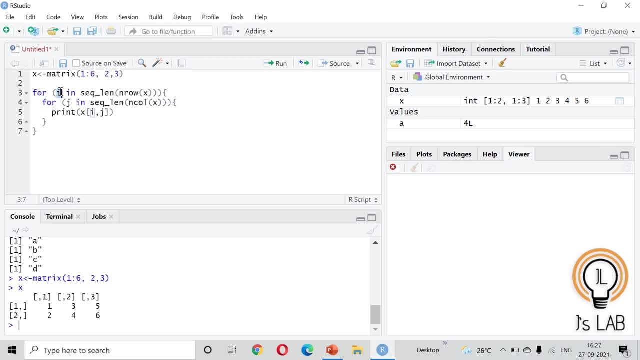 the this values two, okay, i will be two, so it will be looped two times. and j in c, equal length column. three columns are there, so this second for loop will be run for three loops, okay, and it will print the terms, which is i, the term and j each for each iteration. okay, so we'll see. 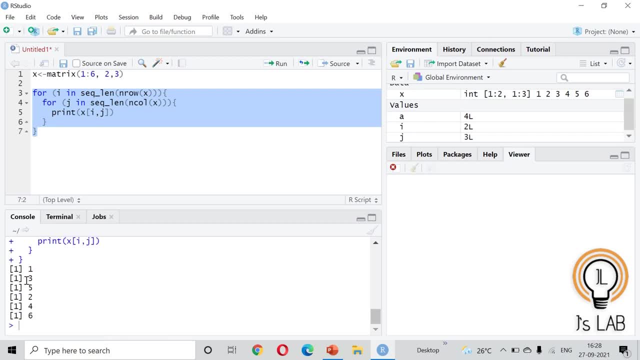 uh, that one. okay, if you run this one you can see one, three, five, two, four, six. okay, if you look closely you can see. first of all it will have the value one, one. so first row, first column, it will be printed. first row, second column, it will be print. then first call third row. so one, three, five. 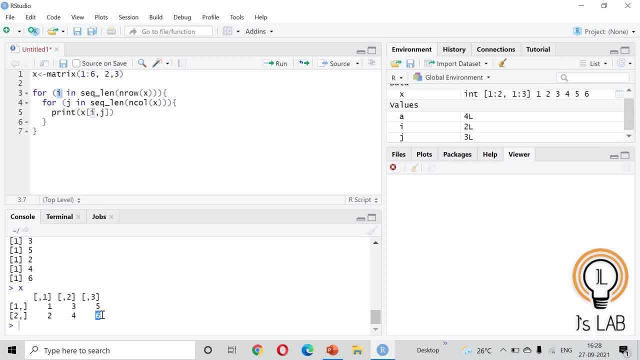 will be printed. then, second row, first column, second row, second column. and second row, third column, two, four, six will be printed. that is the for loop. so we have seen one, a simple for loop, and one for loop inside another form. okay, this for loop will be used, uh, regularly, and it will be. 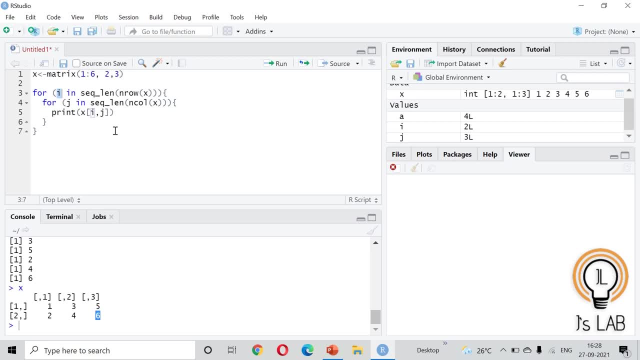 very helpful, helpful while doing the data processing. next one is while loop. okay, while loop, so while. while loop is another major looping construction, r, and the basic idea is that the while is a logical expression and will execute the loop based on that logical expression. if it is true, it. 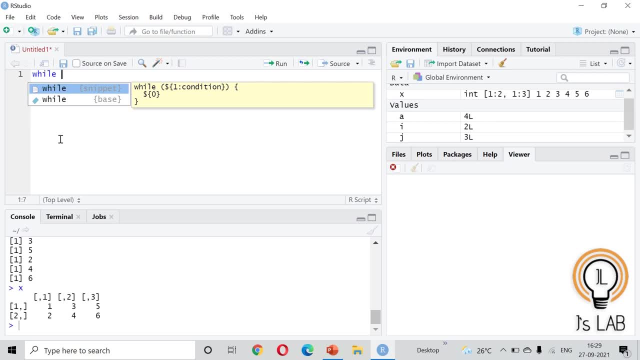 will execute that one, and if it is false, you need to. it will not execute that, and if it is executed, you need to put break or next to break that loop, otherwise it will. if the condition is not provided well, then it will loop for infinite times. okay, so the will look with an example. okay, condition: